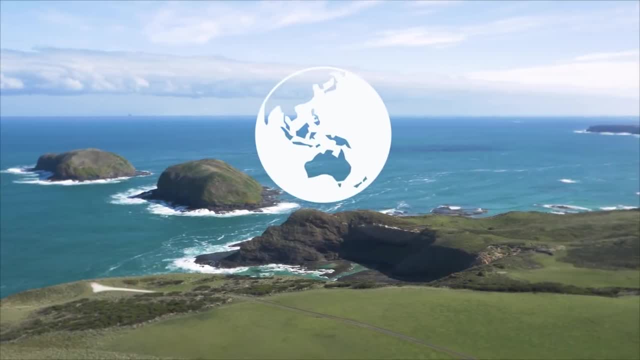 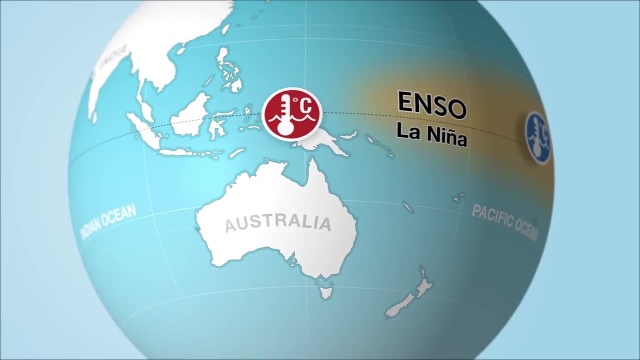 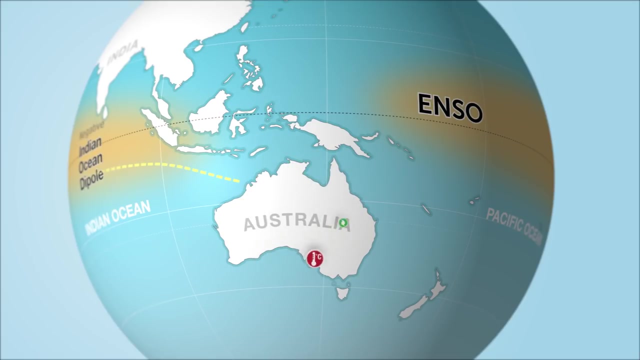 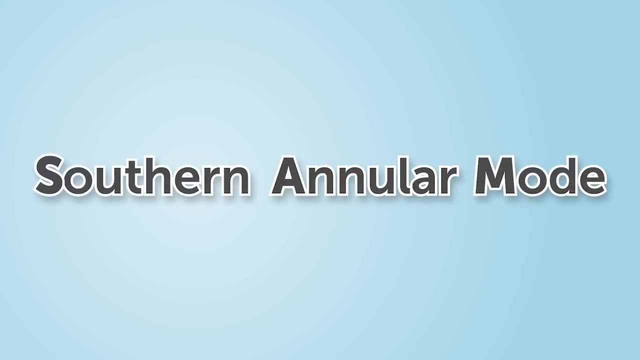 While El Niño, La Niña and the Indian Ocean Dipole are the primary drivers of year-to-year climate variability in Australia, there's a set of secondary drivers that can also play a key role. One of these is the SAM, or the Southern Annular Mode. So what is the SAM? 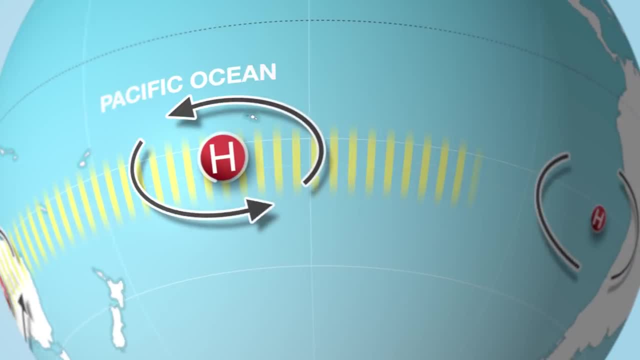 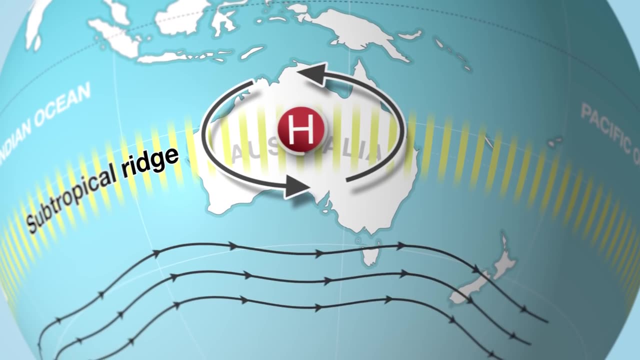 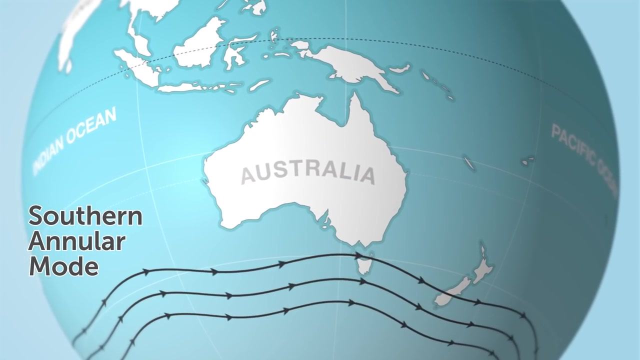 Well. in the Southern Hemisphere a belt of high pressure extends right around the globe. in the subtropics We call this the subtropical ridge. On the southern side of this ridge there are strong westerly winds, the roaring 40s and the furious 50s. SAM refers to the. 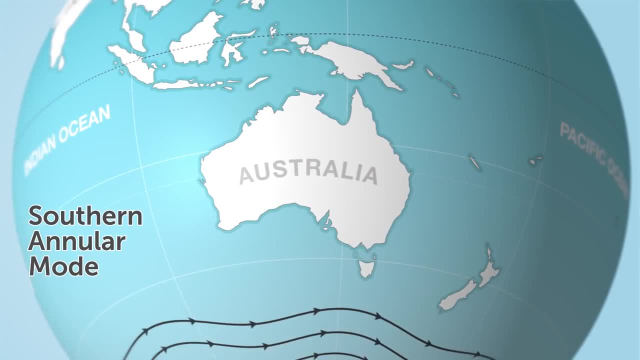 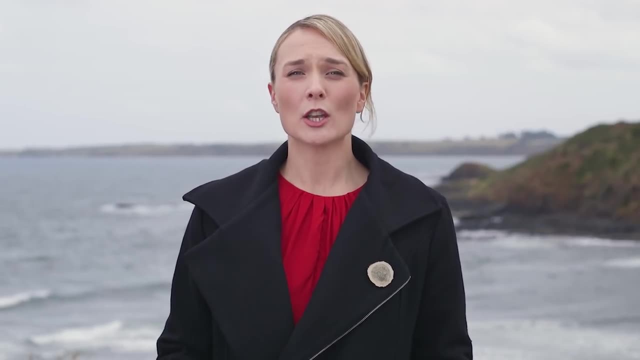 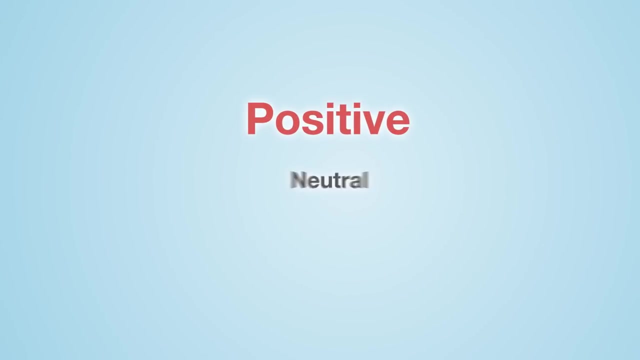 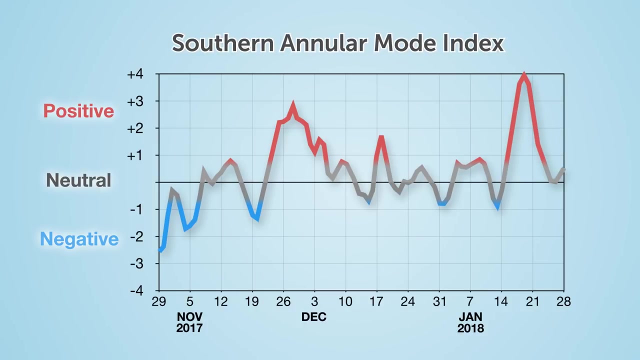 unusual north or south shift of these winds. This shift in the winds away from their normal position can disrupt weather systems around the Southern Hemisphere, including those that bring rainfall to southern Australia. SAM varies between three phases: positive, neutral and negative. These phases last around two weeks, but can sometimes hang around even longer. 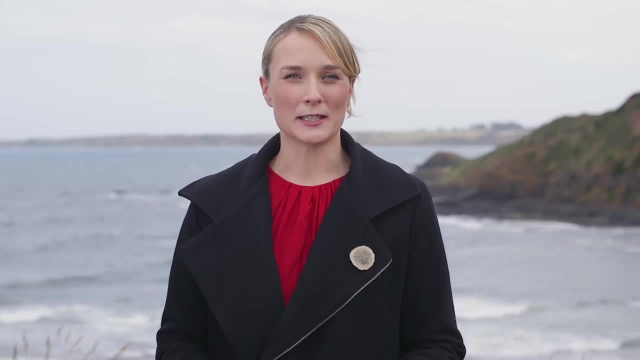 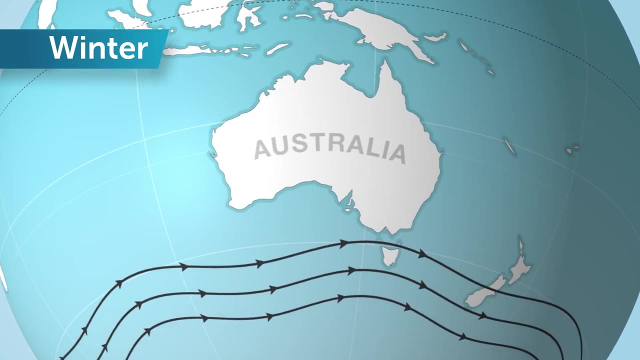 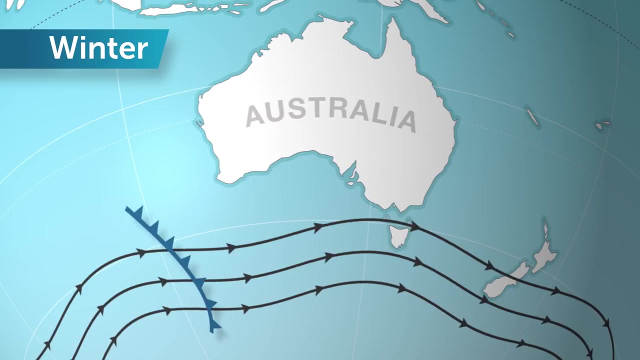 SAM's influence on Australian weather patterns varies during the year. Winter is the time that has the greatest impact across southern Australia. Typically during winter, the top of this belt of westerly winds is located over southern Australia. This means cold fronts are drawn up from the south and can cross the Australian coast, bringing normal. 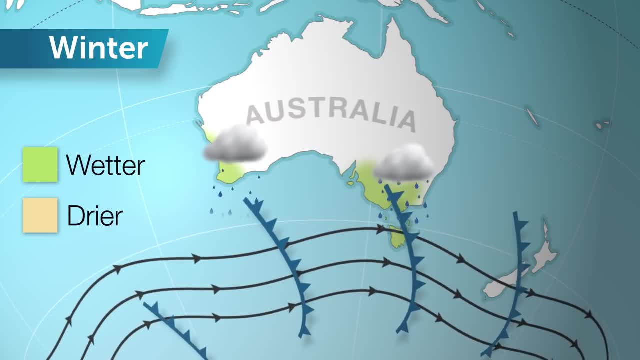 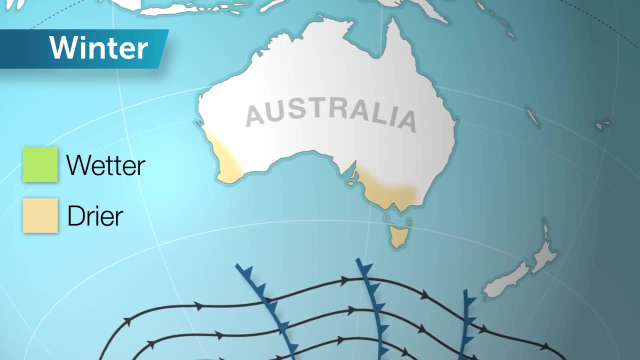 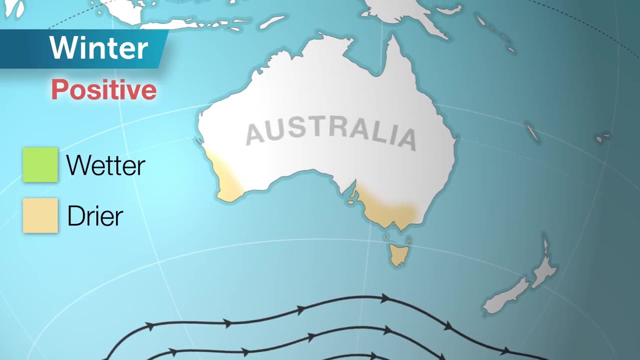 winter rains. But if these winds shift towards Antarctica, the rain-bearing systems also head south. This means fewer fronts and drier conditions for southern Australia. This shift south in the weather systems is called a positive SAM, But a positive SAM can also mean parts. 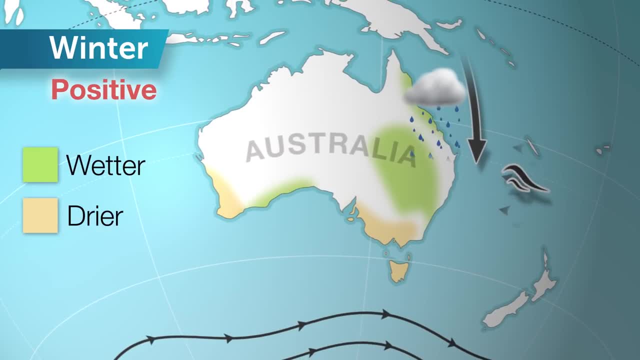 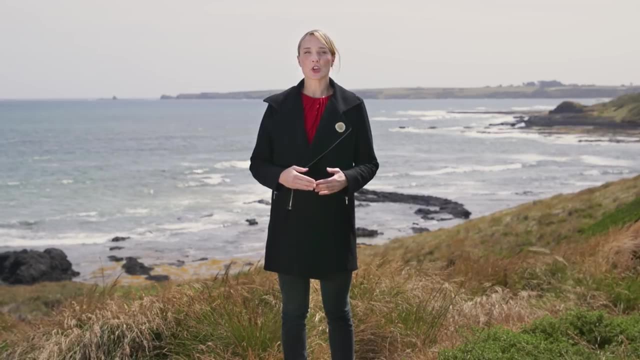 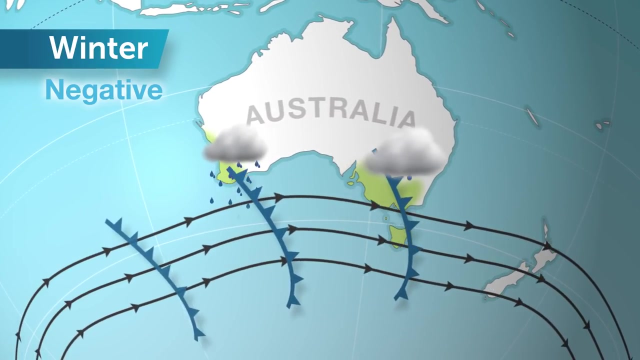 of the east coast get wet, as it draws more tropical air southwards and allows more onshore easterly winds than normal. The opposite is a negative SAM, which occurs when the westerly winds are further north than usual. This allows more wet and cold weather to be drawn up from the south. A negative. 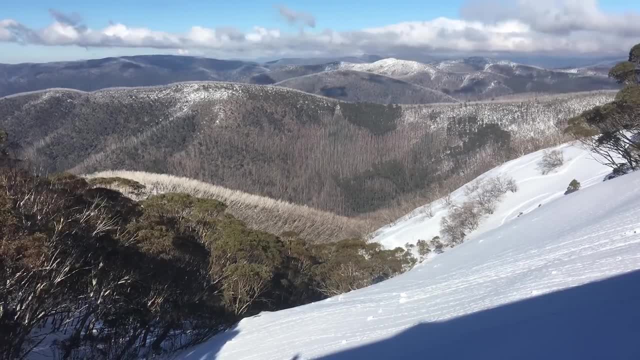 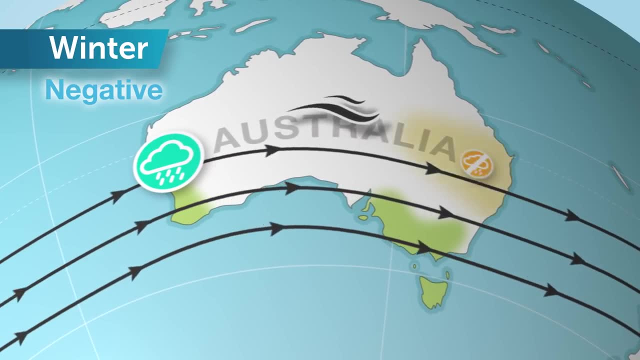 SAM in winter can also help bring good snowfall to the Alps, But if it moves too far north, the westerlies blow right across the continent, meaning the air is wet in the west but dry by the time it reaches the east coast.